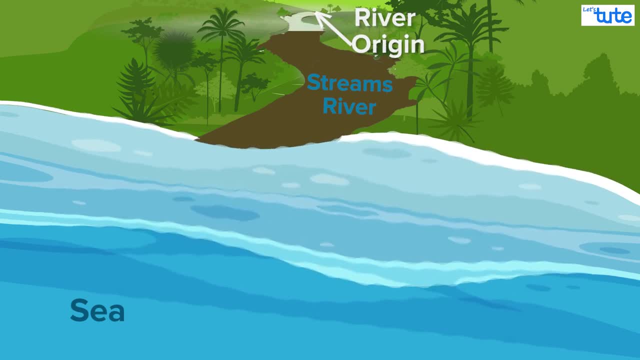 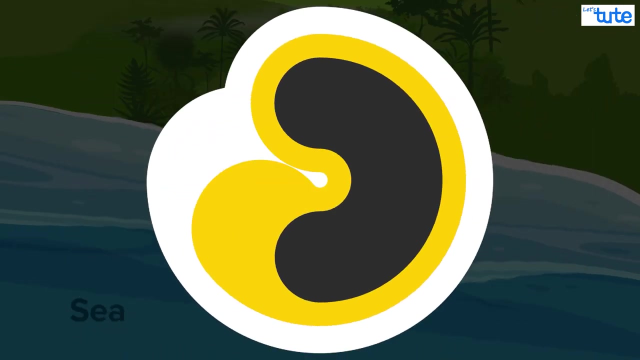 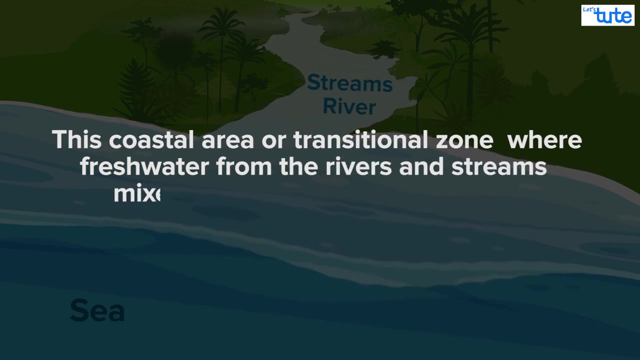 The rivers originate from a particular point, then flows through different regions and finally meet the sea. The region at this point of intersection forms an ecosystem. Let's explore the same in this session: The coastal area or transitional zone, where fresh water from the rivers and streams mixes. 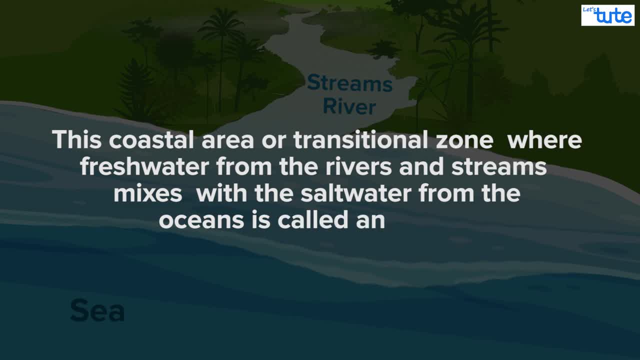 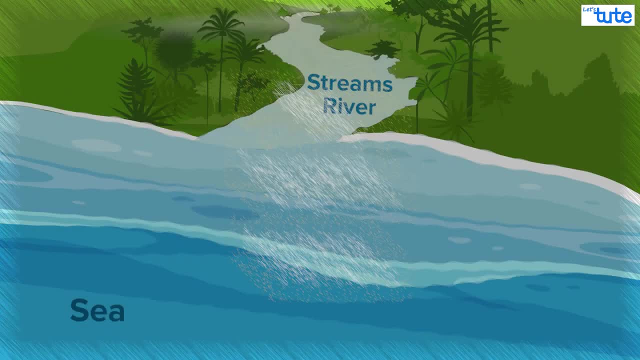 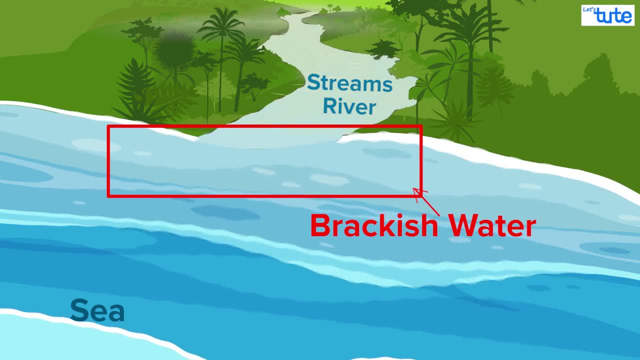 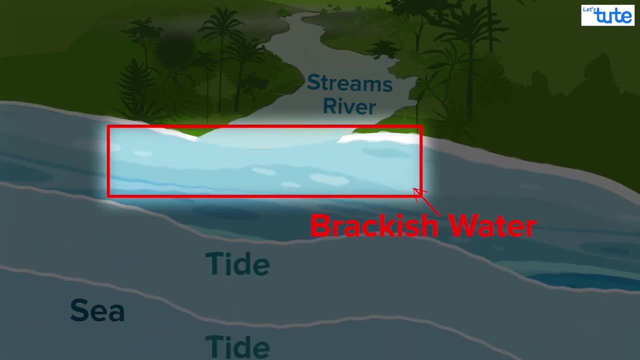 This region is called brackish water. This is because the salt water from the sea enters this region by the action of the tide, But it is diluted by the fresh water coming from the streams and rivers. So the water here is neither completely salty nor fresh. 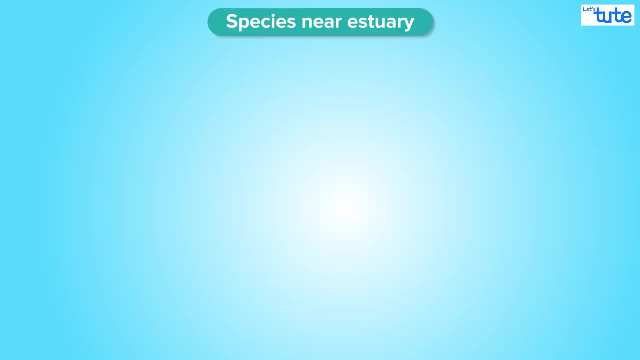 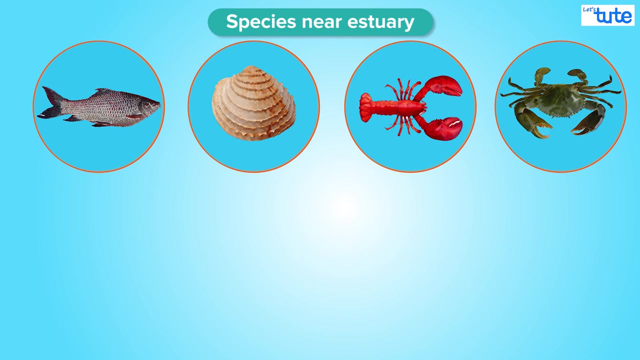 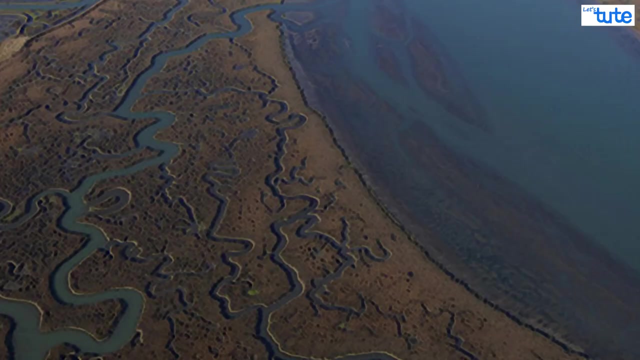 Estuaries are home to a variety of organisms like fishes, shellfishes, lobsters, crabs, sea birds, goose, marine worms and many different reptiles. Sometimes these estuaries are full of dead, decaying organisms. They are marshy and the soil is nutrient rich. Estuaries are often called nurseries of the ocean. Can you think why is it so? This is because many fishes lay eggs in the estuaries and the abundant plant protects these eggs. This is because many fishes lay eggs in the estuaries and the abundant plant protects these eggs. 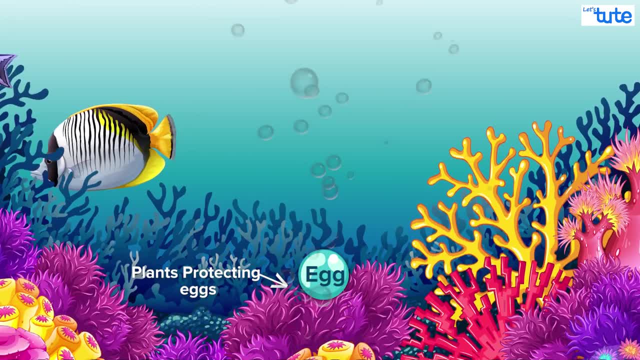 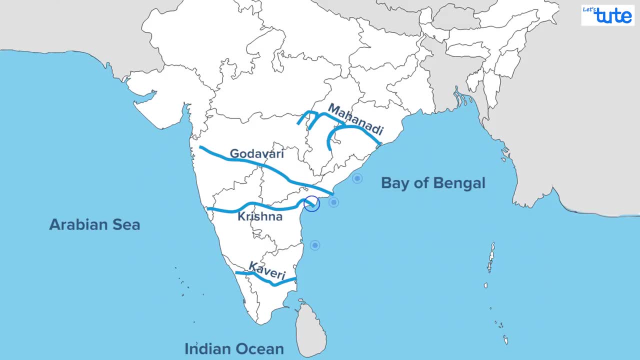 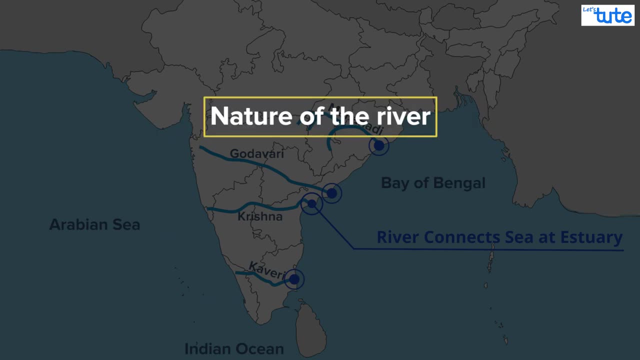 This is because many fishes lay eggs in the estuaries and the abundant plant protects these eggs, Thus nurturing new lives. Do all rivers form estuaries, you might ask? Well, most rivers that connect the sea form estuaries at the mouth. This also depends on the nature of the river, that is, whether 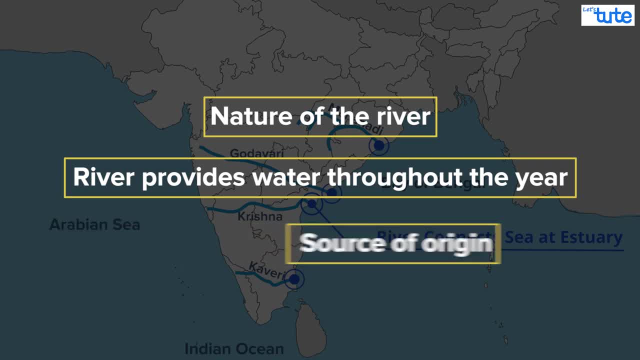 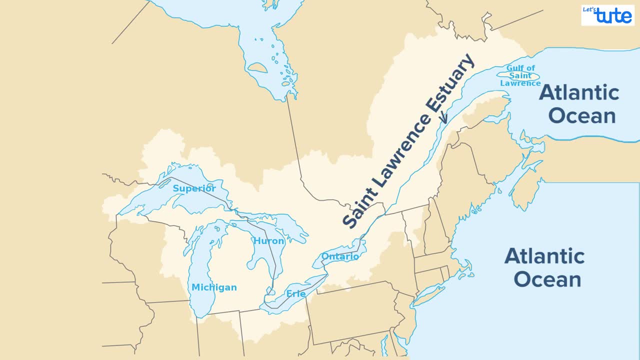 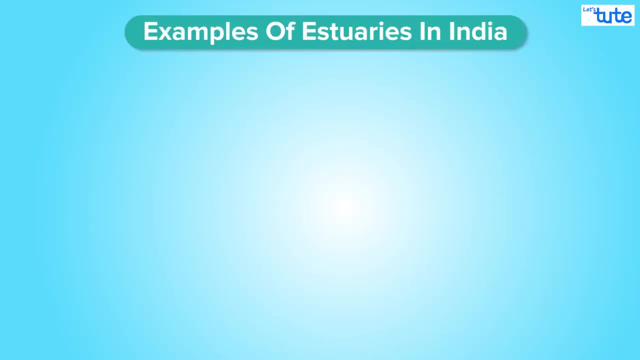 the river provides water throughout the year, the source of it, etc. The world's largest estuary is the Gulf of St Lawrence River that connects the Great Lake to the Atlantic Ocean. Some examples of estuaries in India are the Thane Creek in. 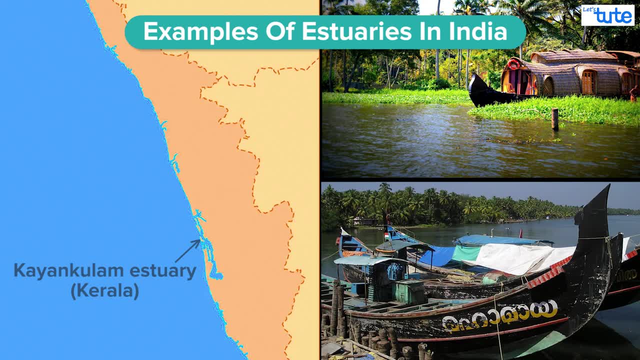 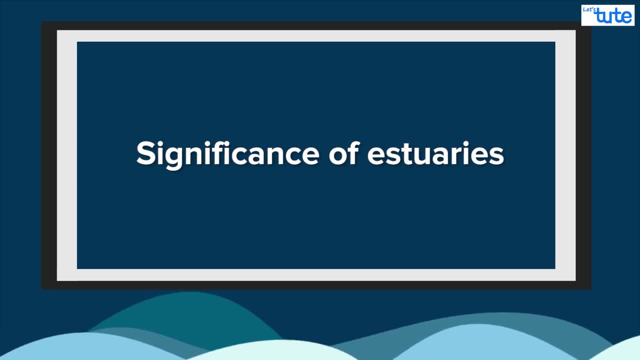 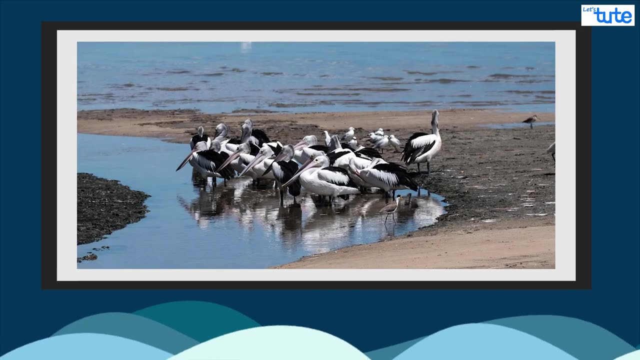 Mumbai Baga Creek, the Kayamkulam Estuary, etc. The estuaries have a lot of significance Considering the environmental aspect. they are breeding and nesting grounds for many organisms. They have ecological significance. They control pollution by filtering and absorbing the waste canals. They are also a source of